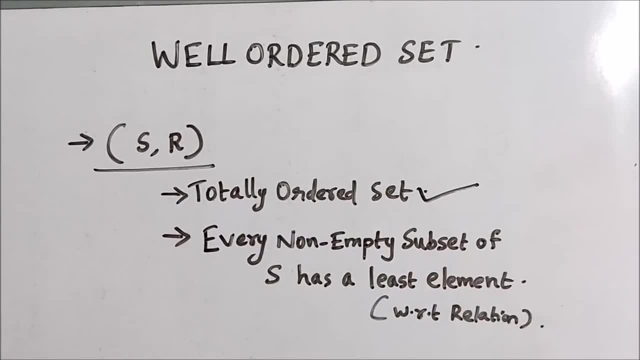 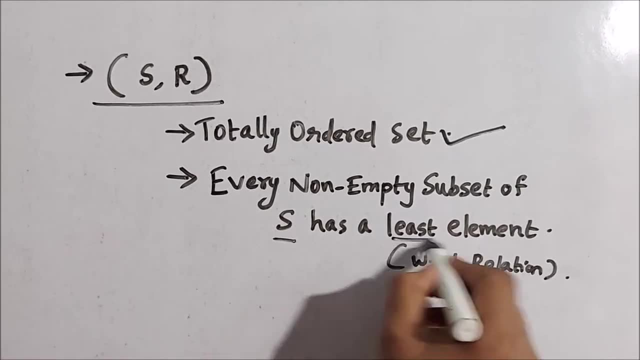 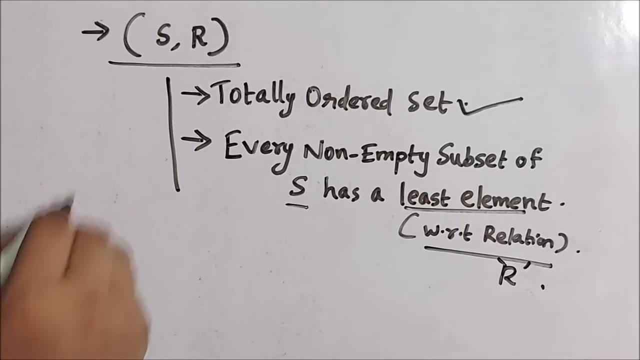 R should be a totally ordered set. Also, if you take every non-empty subset of the set S, it has a least element with respect to the relation R. If these two conditions are met, then the set S, together with the relation R, is called a well-ordered set. 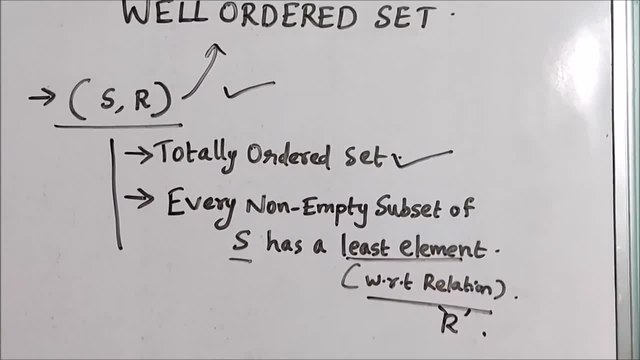 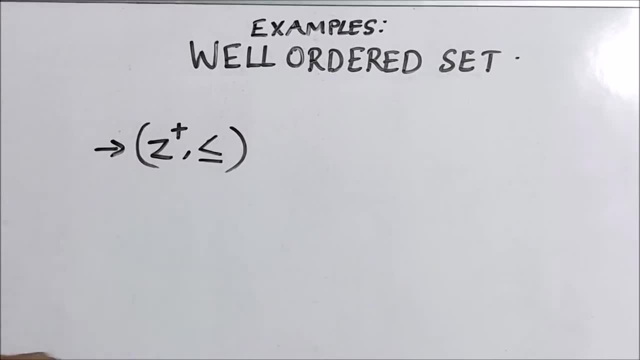 We will see some examples of well-ordered set. Then we will understand it more clearly. So let's consider the set of positive integers together with the less than or equal to relation. So the set of positive integers together with the less than or equal to relation. 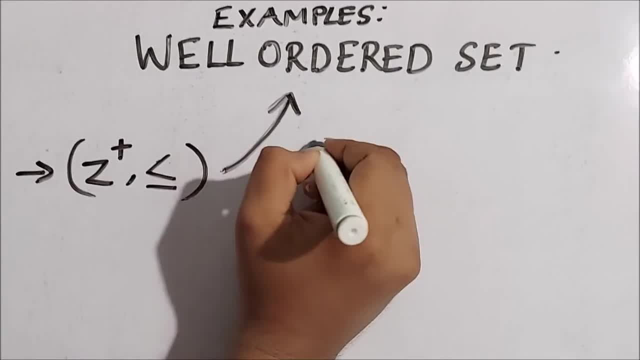 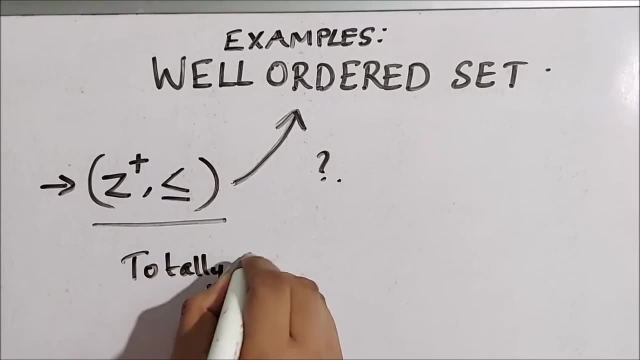 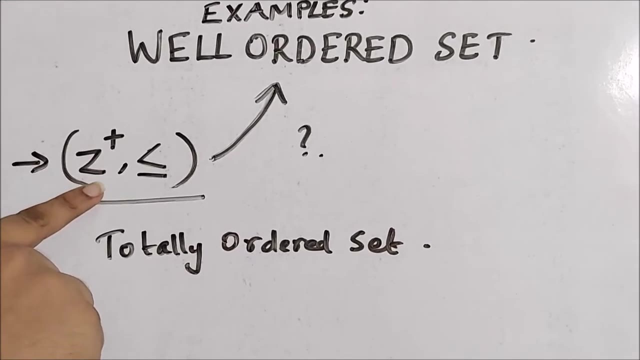 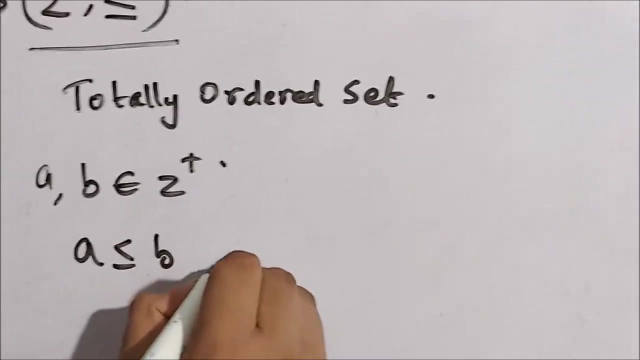 whether that is a well-ordered set or not. that is the question, okay, so first of all we have to understand this is a totally ordered set, okay. one thing is that if you take any two elements in the set of positive integers- a, comma, b- if you take, we know that either a is less than or equal to b, or b is less than or equal. 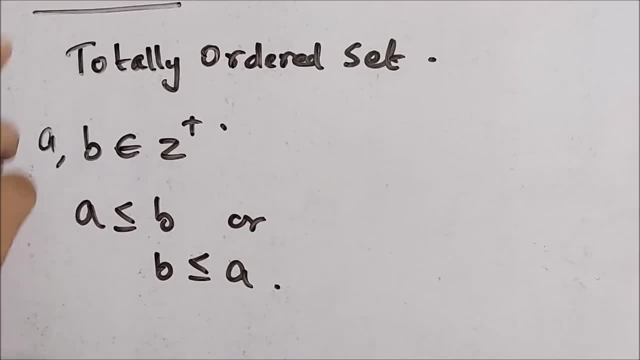 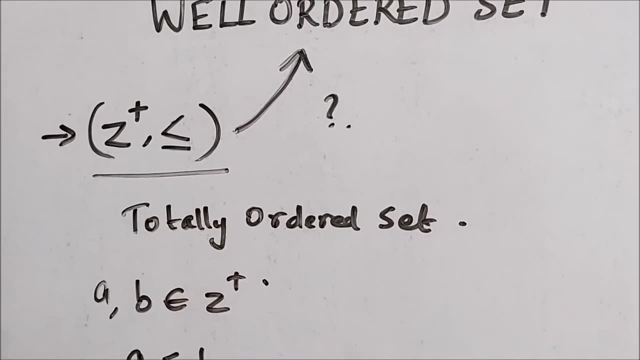 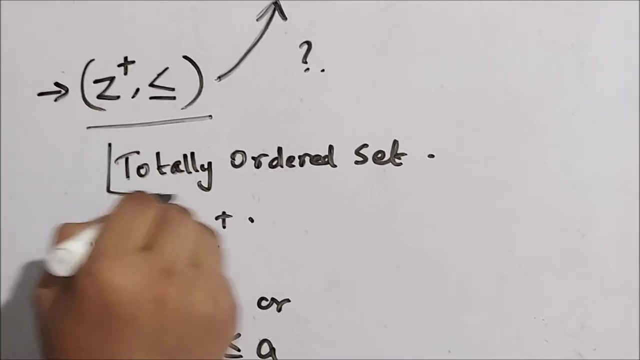 to a. that means every pair of elements in the set of positive integers are comparable. okay, and also the less than or equal to relation defined on this set is also a partial ordering relation. that is the reason why this set set plus comma less than or equal to is a totally ordered set. 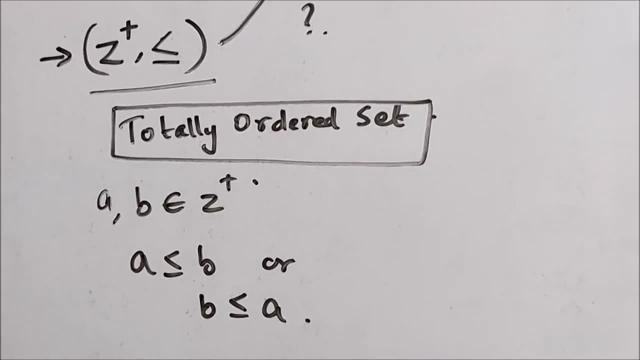 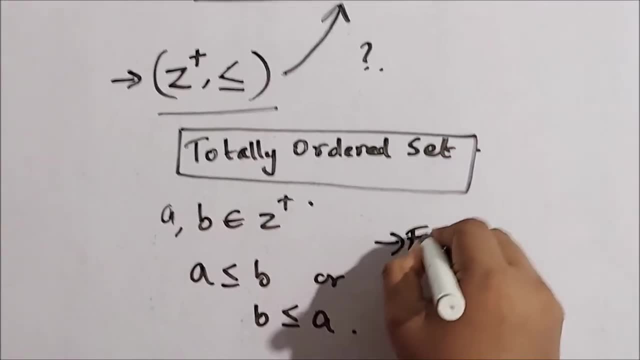 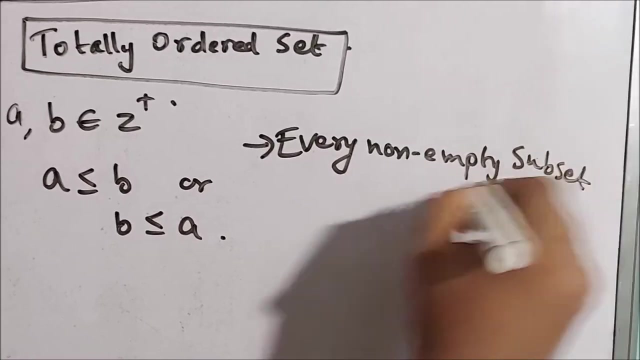 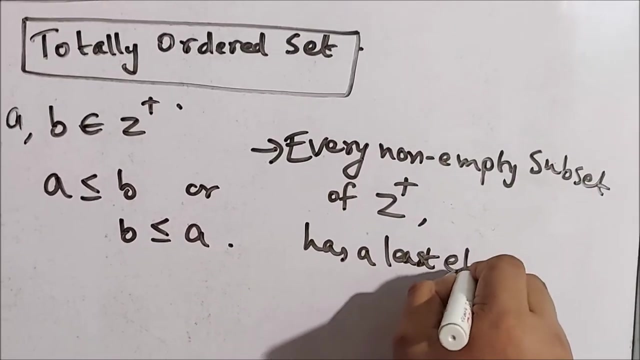 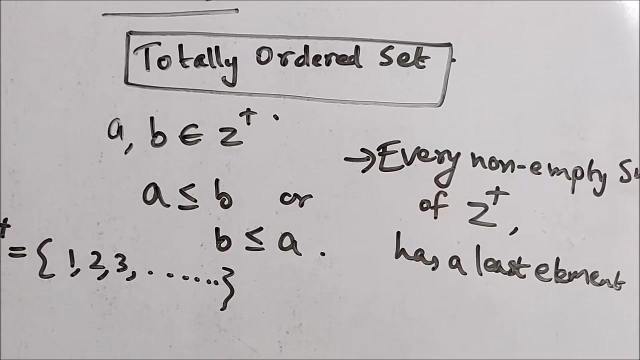 okay. now we also have to check the second condition for this set to being a well-ordered set. we also have to check that whether every non-ambiguous subset, right, every non-empty subset of set plus has a least element or not. okay, okay, so the set of positive integers is an infinite set, right? basically. so now what we are. 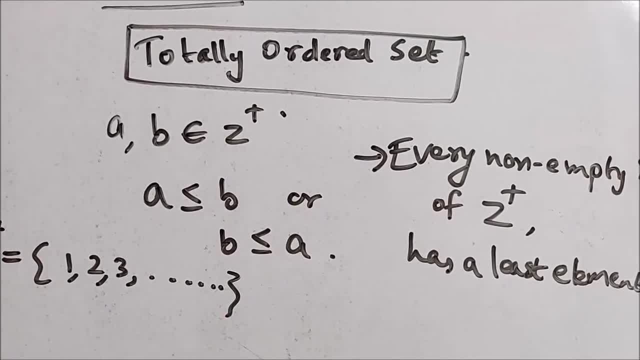 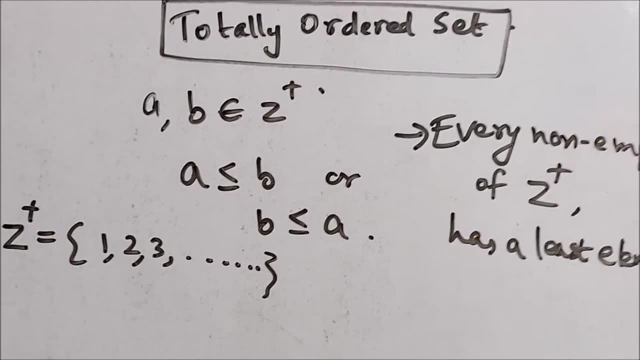 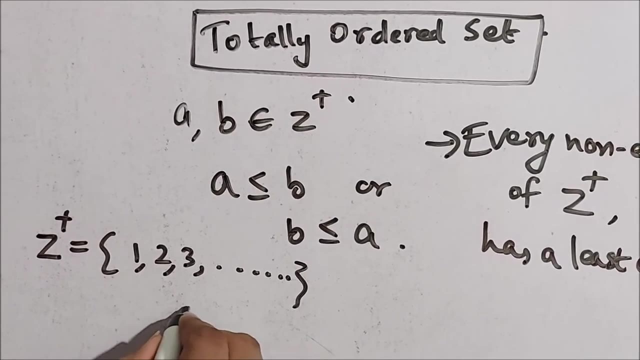 claiming is that you take any non-empty subset of set plus, meaning that you take a subset of set plus which have at least one element in it. right then, we have a least element, right so, since the relation is less than or equal to always, if suppose the subset you are taking is. 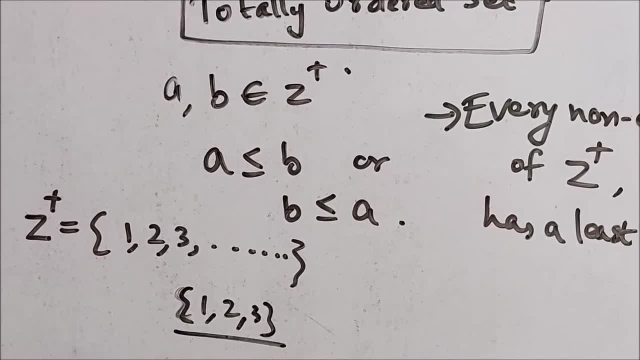 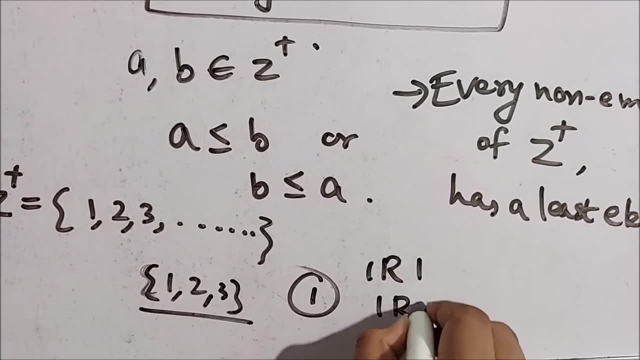 1, 2, 3. as an example, the subset you are taking is 1, 2, 3. there is a least element, which is 1, because one is related to 1, one is related to two, one is related to three and hence one is the least element here, as one is less than or equal. 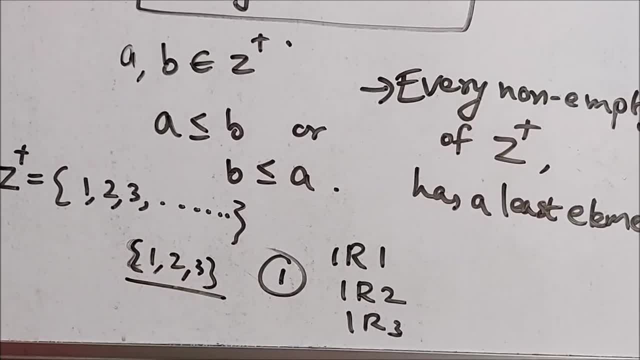 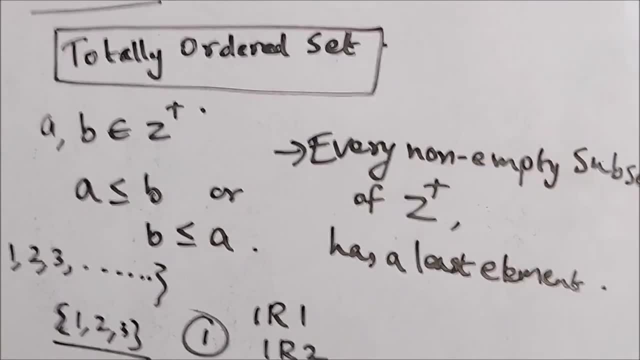 to one. a second set possesses much shorter set than or equal to one than. one set possesses less than Д is less than 2 and 1 is less than 3.. So the thing is that if you take any non-empty subset of the set of positive integers, there will be a least element when the relation is less. 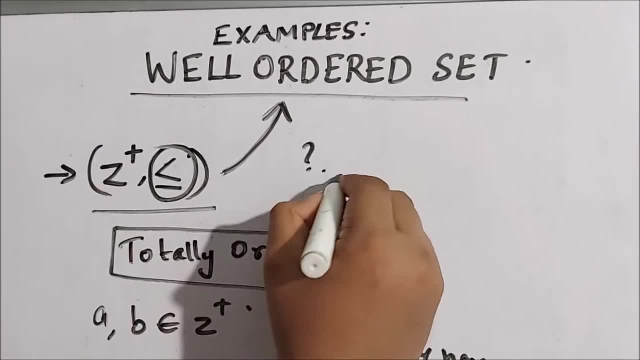 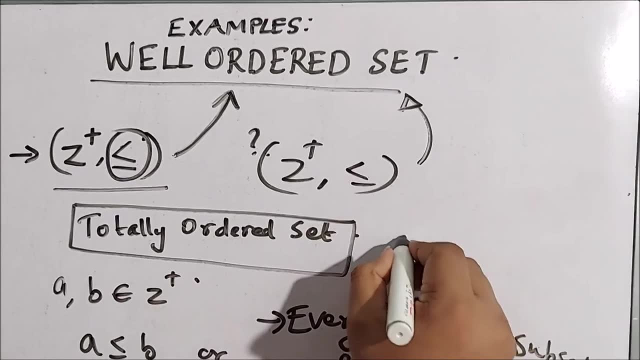 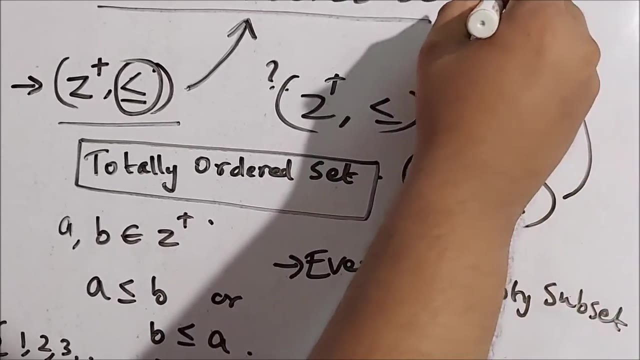 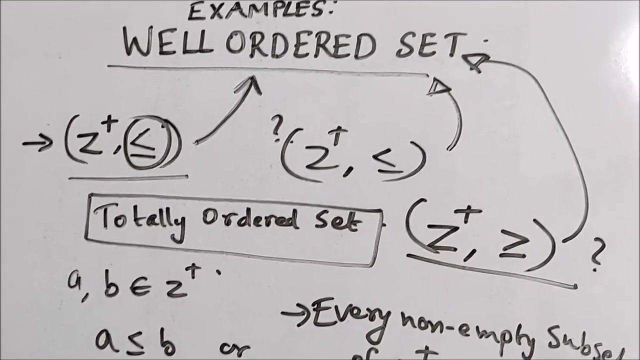 than or equal to, right. That's why set plus comma, less than or equal to is a well-ordered set. okay, Now what about this set? You take set plus comma, where the relation is greater than or equal to. Whether this is a well-ordered set. Okay, Think about it for a moment. We. 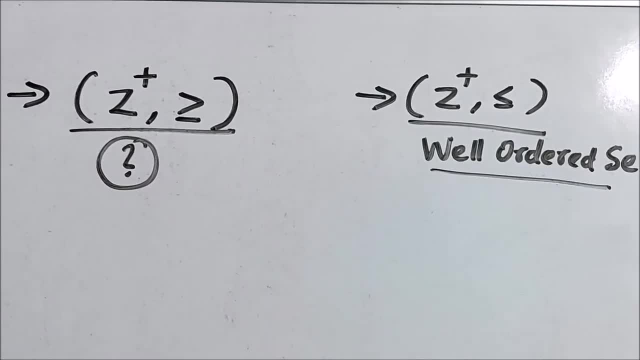 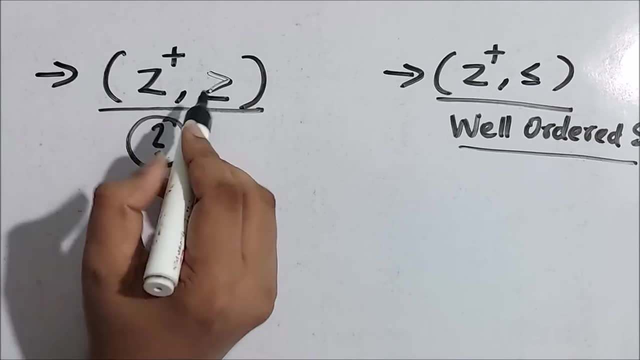 know that set plus comma less than or equal to is a well-ordered set. We have seen that. Now the question was whether this set the set of positive integers together with the relation greater than or equal to. okay, Whether this is a well-ordered set or not, Okay So 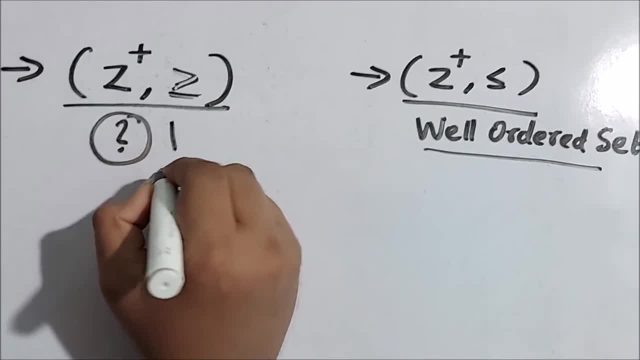 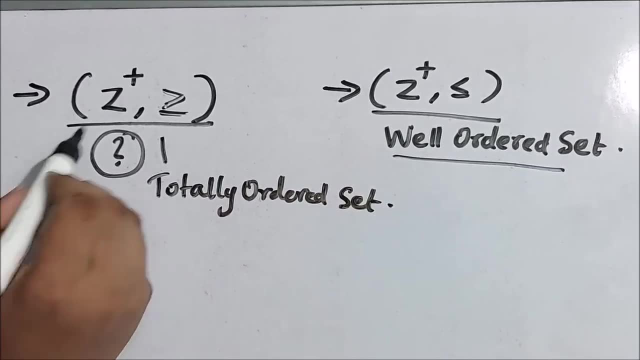 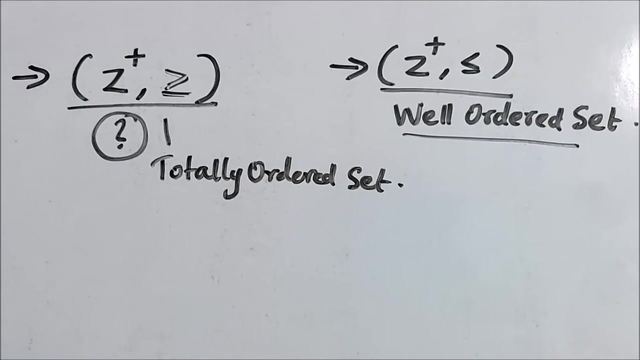 basically, we can see that this is a Totally ordered set right. Every pair of elements belonging to a set of positive integers is comparable with respect to this relation. That is clear, That we know. Also, we know that the greater than or equal to relation defined on the set of integers we have seen, 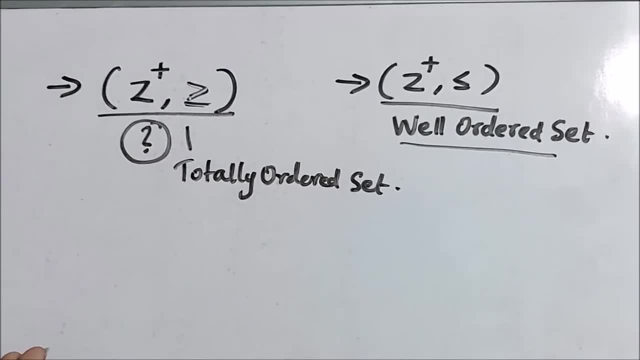 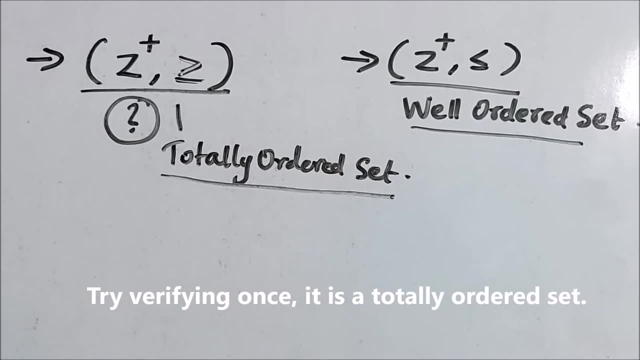 that that was a partial ordering relation or that was a partially ordered set. So, again, this is going to be a totally ordered set, But the question is Whether it satisfies the second property for it to become a well-ordered set. What was? 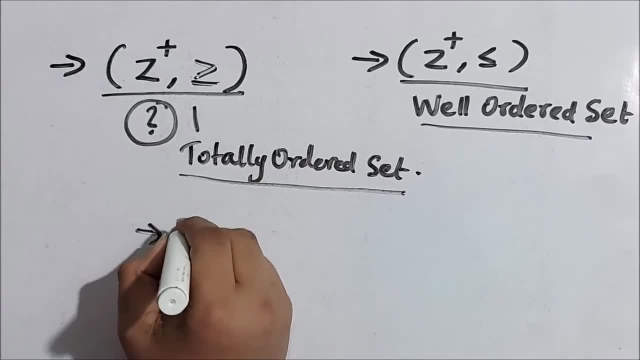 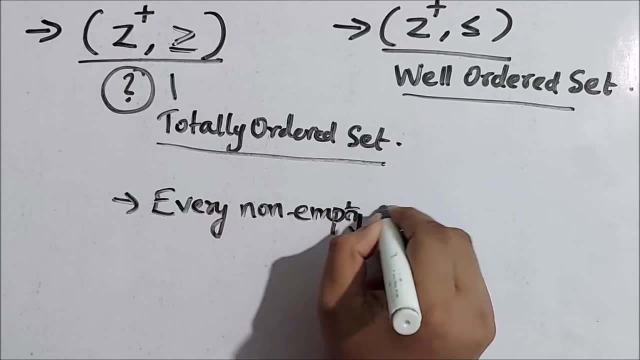 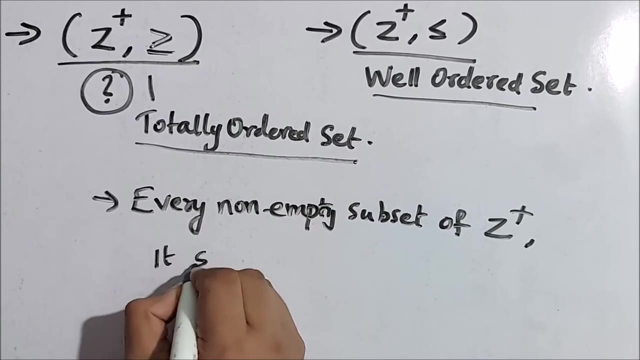 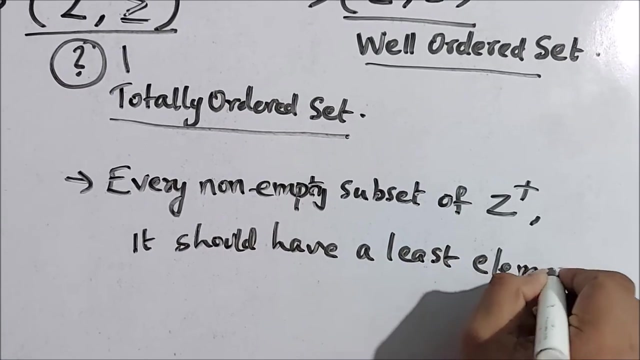 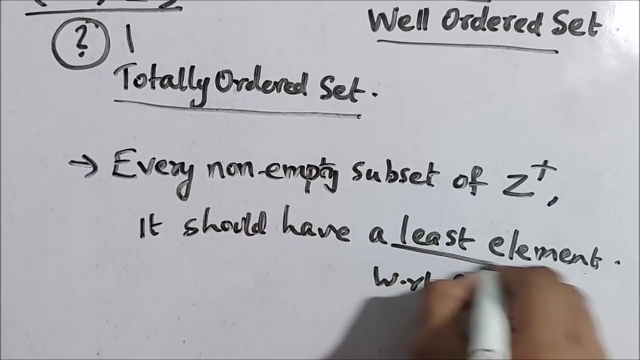 the second property. It has to be the case that you take every non-empty subset right, Every non-empty subset of the set of positive integers. it should have a least element right. That was the Second property with respect to the relation. So when we say that it should have a least, 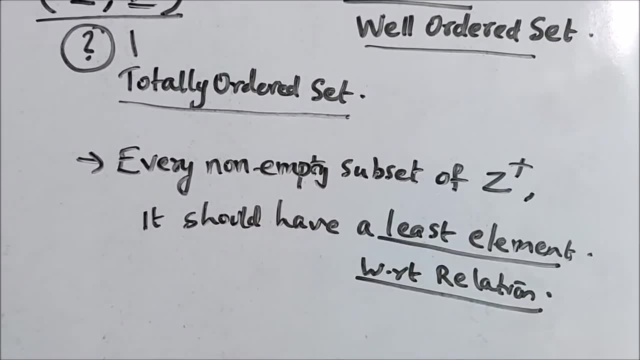 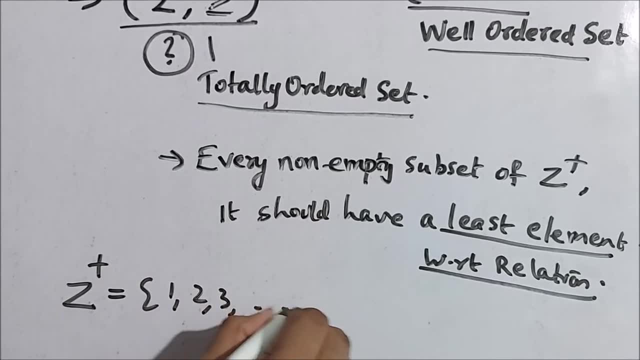 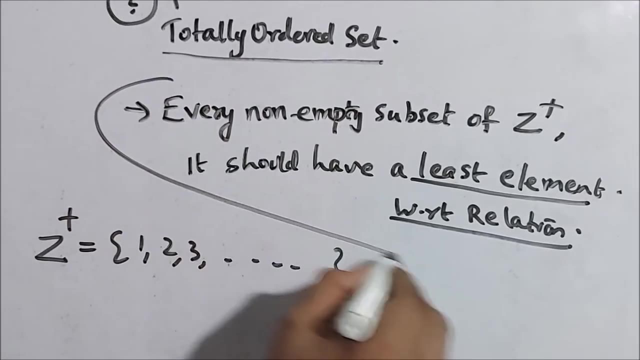 element. it is with respect to the relation. So the relation here is the greater than or equal to relation and the set plus the set is the set of positive integers. okay, This is an infinite set. okay, Now we are trying to prove that this is not the case. 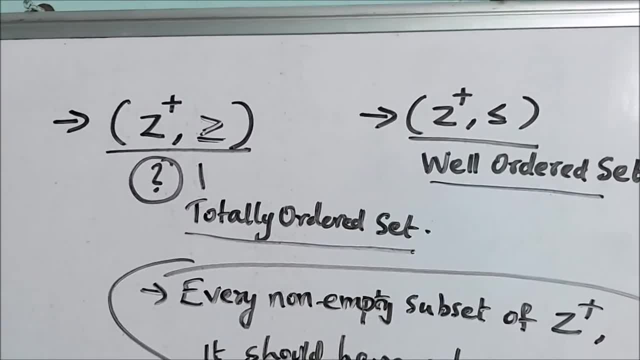 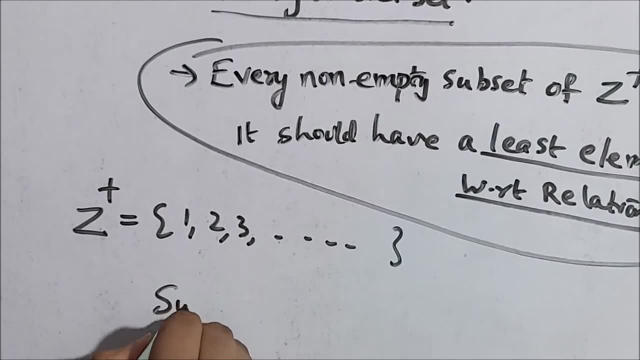 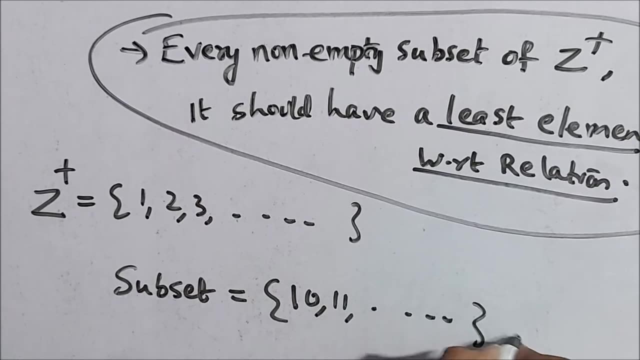 for the relation greater than or equal to right. Okay, So let's take a non-empty subset. here We are proving with a counterexample. So let's say, the subset that we took was 10 comma, 11 comma, 2 infinity. okay, This was a subset. 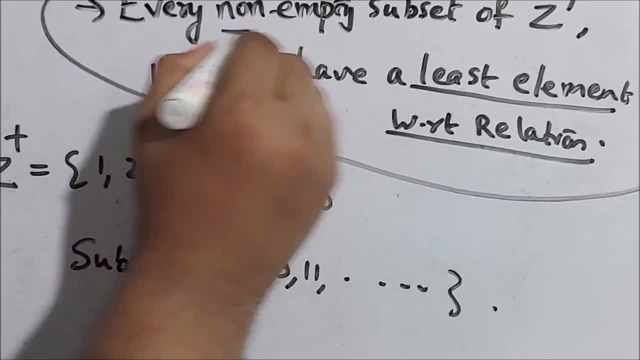 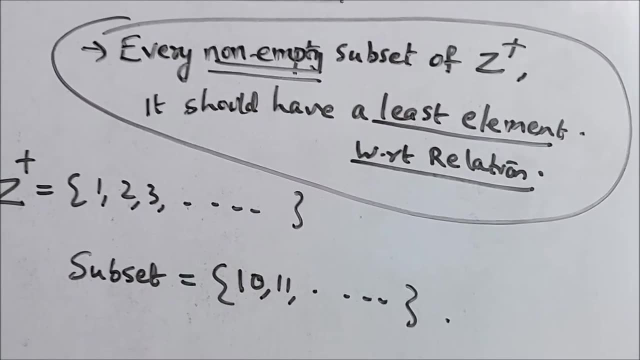 It's an infinite subset, but it's a non-empty subset, right Non-empty subset- of a set of positive integers, Whether it has a least element or not. Of course it has a least element: It has a set of positive integers. 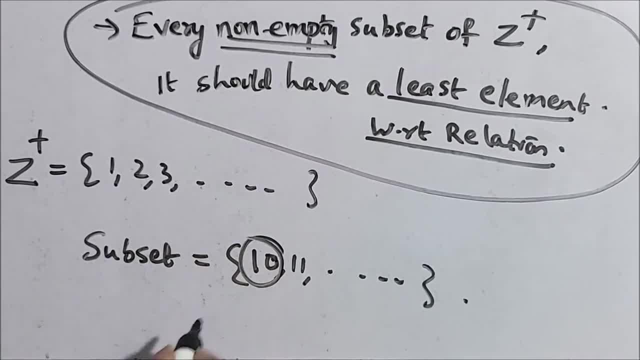 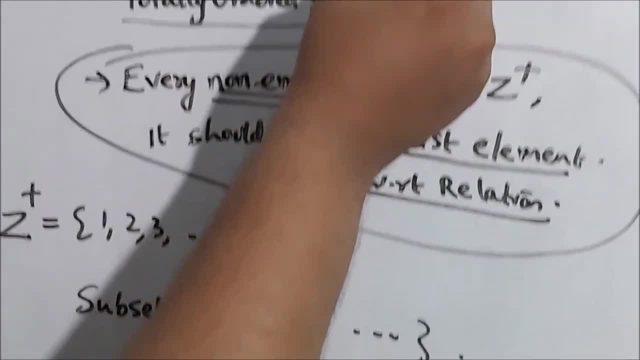 It has a set of positive integers. Of course it has a least element 10, but it is with respect to the relation less than or equal to right. So with respect. so if set plus comma less than or equal to, we already 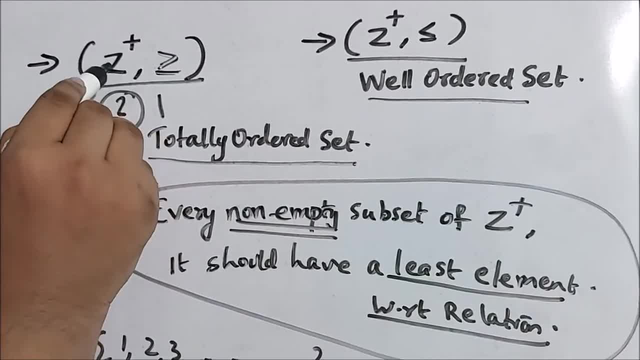 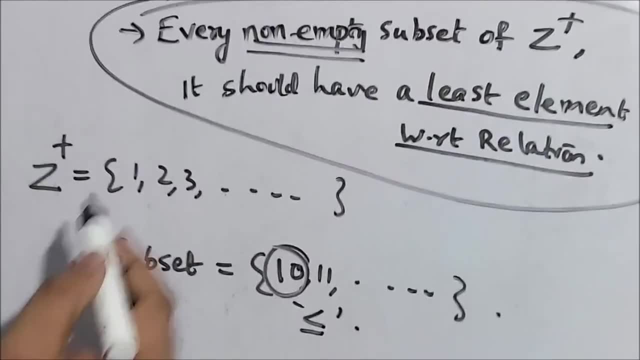 know that it is a well-loaded set, But the question here is whether set plus comma greater than or equal to whether it is a well-loaded set or not. That is the question. okay, And you take a non-empty subset of the set of positive integers and you prove that it doesn't. 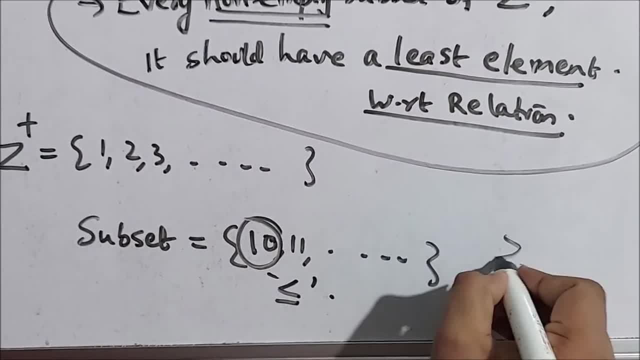 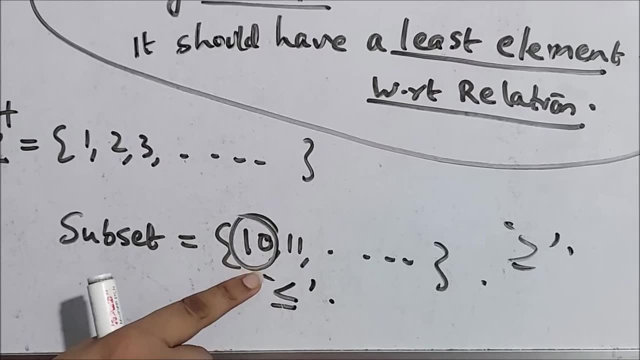 have a least element with respect to the relation, Provide that the relationship of all the elements of any set is less than or equal to. So obviously this subset has the least element with respect to less than or equal to, because 10 is less than or equal to all the elements in the set right. 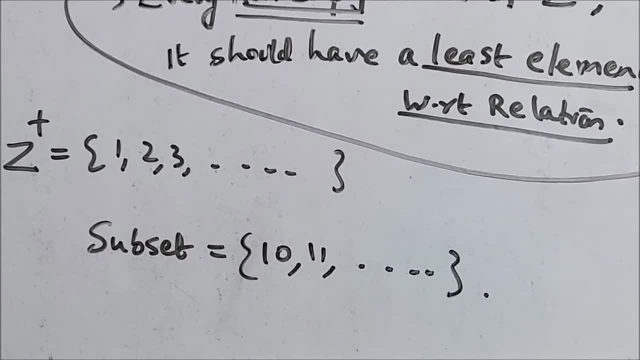 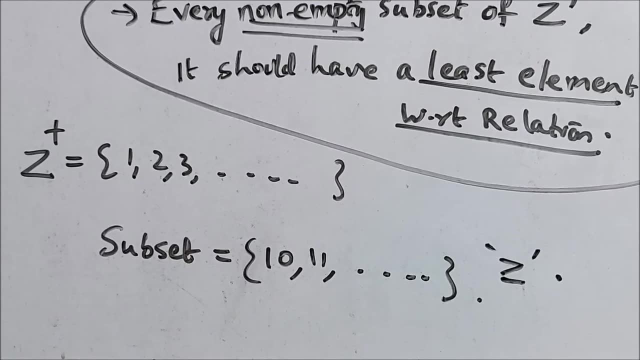 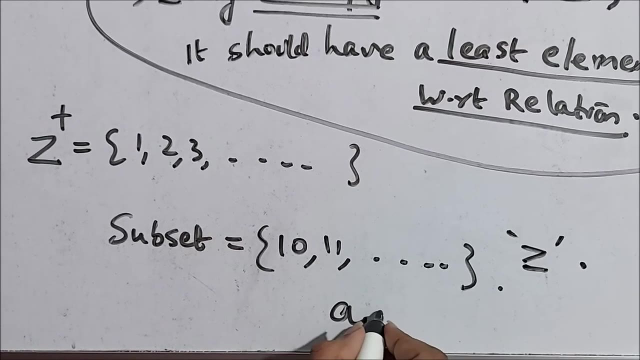 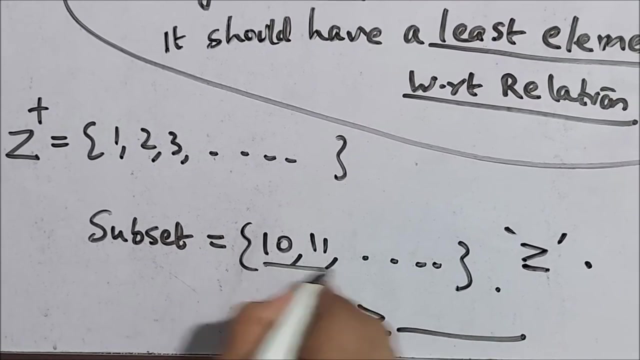 Okay. So now our question is whether this subset has a least element with respect to the greater than or equal to relation, Meaning that if there was a least element- A Okay- In this subset, it should be the case that A is related to every element in this set. 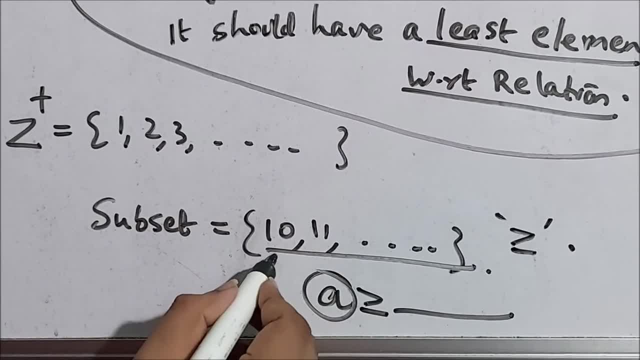 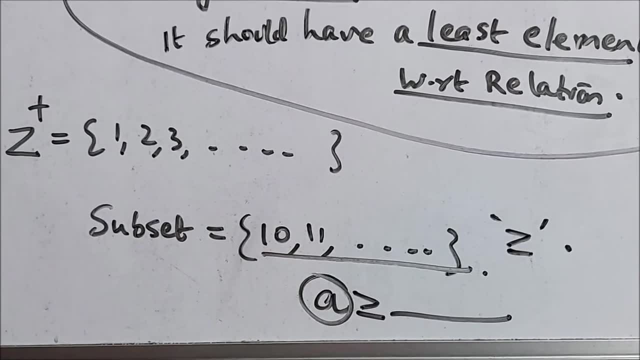 Okay, So can we say an A which is greater than or equal to every element in this set? That is the least element here and not the 10.. 10 is the least element with respect to the less than or equal to relation and not with the greater than or equal to relation.